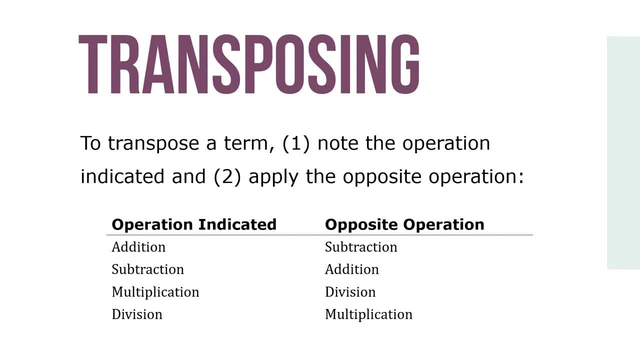 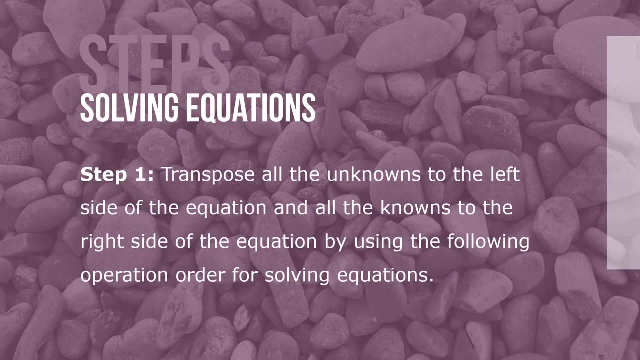 of the equation as follows: If the operation indicated is addition, use subtraction. If it's subtraction, use addition. If it's multiplication, use division. And if it's division, use multiplication. Here are the steps for subtraction, For solving equations and proving the solution: Step 1. Transpose all the unknowns to the 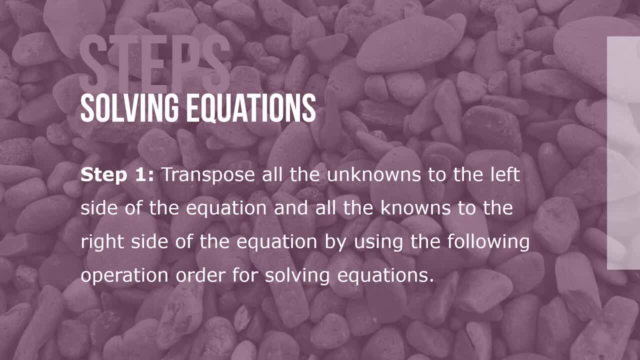 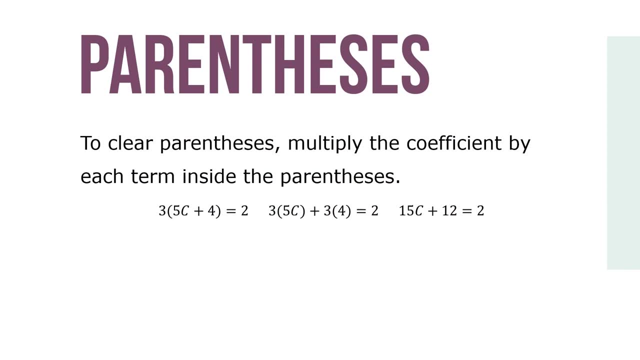 left side of the equation and all the knowns to the right side of the equation by using the following operation order for solving equations: Parentheses, if any, must be cleared before any other operations are performed. To clear parentheses, multiply the coefficient by each term inside the parentheses. So if our equation is 3, parentheses 5, we have 3. 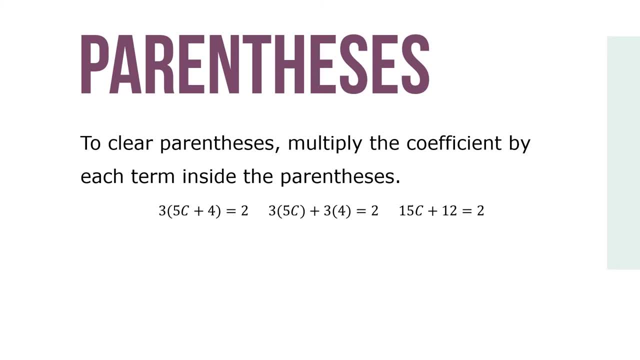 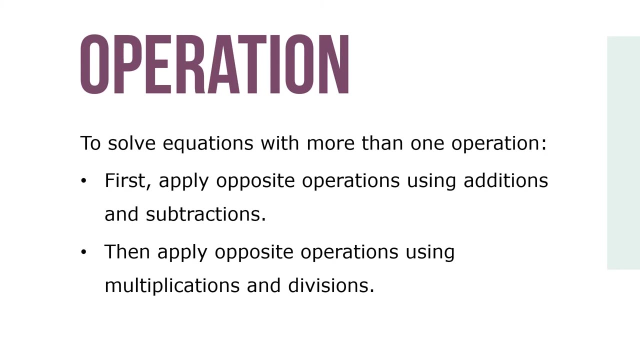 parentheses 5c plus 4 equals 2.. Then we convert 3 parentheses 5c plus 3 times 4 to equal 2.. So 15c plus 12 equals 2.. To solve equations with more than one operation, first apply opposite operation using additions. 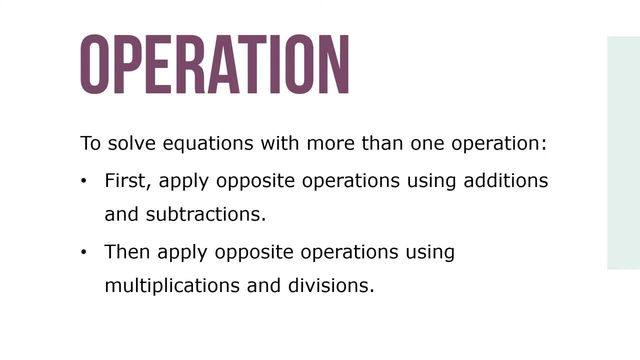 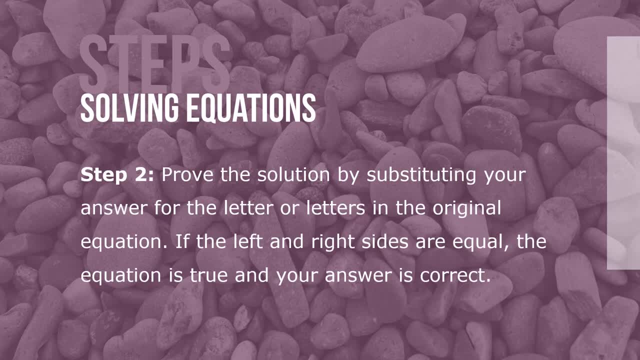 and subtractions. Then apply opposite operations using multiplication and division. Step 2. Prove the solution by substituting your answer for the letter or letters in the original equation. If the left and right sides are equal, the equation is true and. 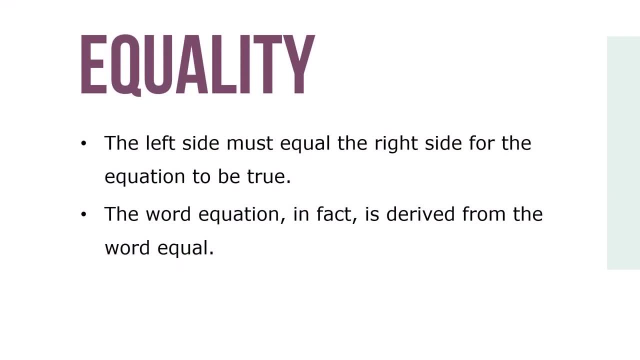 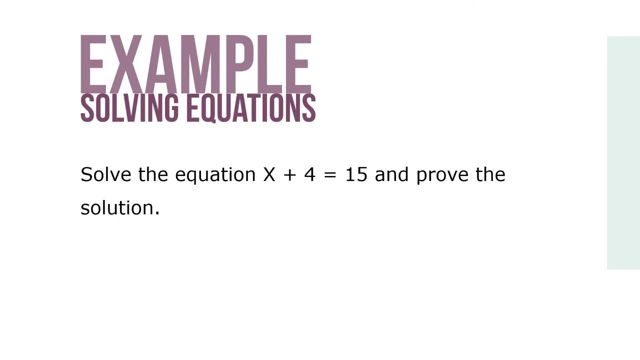 your answer is correct. Remember, an equation is a statement of equality. The left side must equal the right side for the equation to be true. The word equation, in fact, is derived from the word equal. Let's use an example: Solve the equation x plus 4 equals 15 and prove the solution. 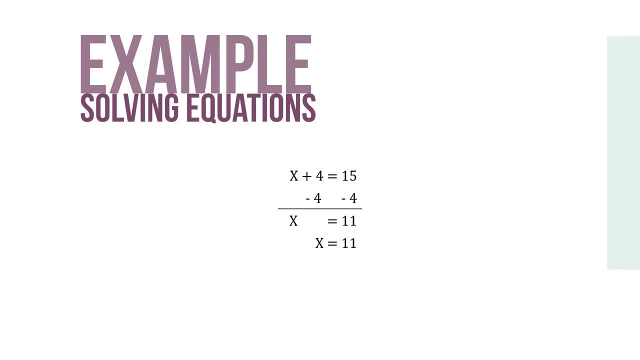 The equation x plus 4 equals 15 indicates addition plus 4.. To solve for the x, apply the opposite operation: subtraction, Subtract 4 from each side. Now for proof. The solution can be easily proven by substituting our answer 11, for: